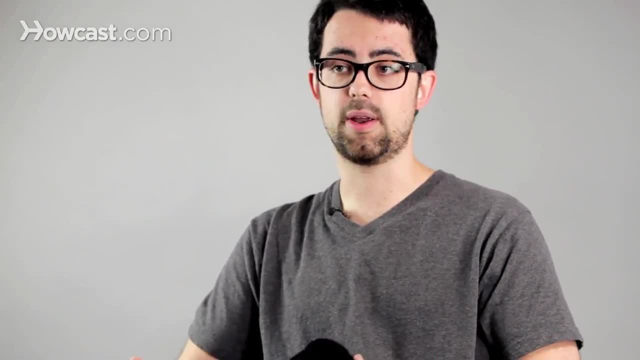 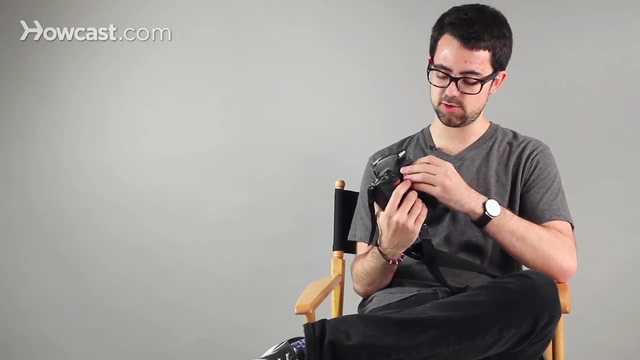 is going to have a lot of distortion, but you're going to get a lot in the frame. So, like I said, all digital SLR cameras need a lens to take pictures. otherwise you just have a mirror and a sensor in there. Simply take your lens. 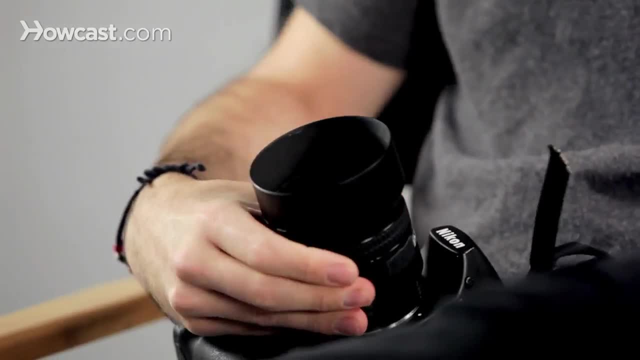 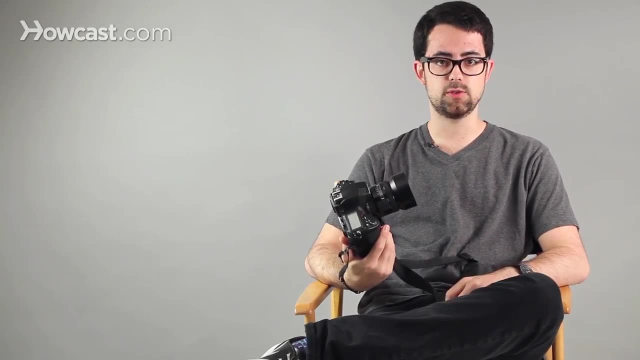 Remove the caps and attach it on, And that's one of the nice things about digital photography with an SLR is you can switch your lenses out, whereas if you were using a point and shoot camera, the lens is fixed and you obviously can't remove it. 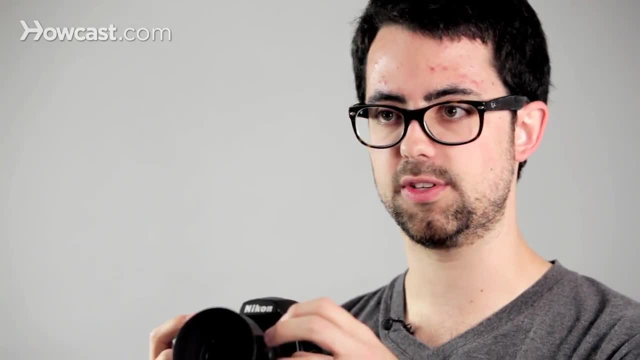 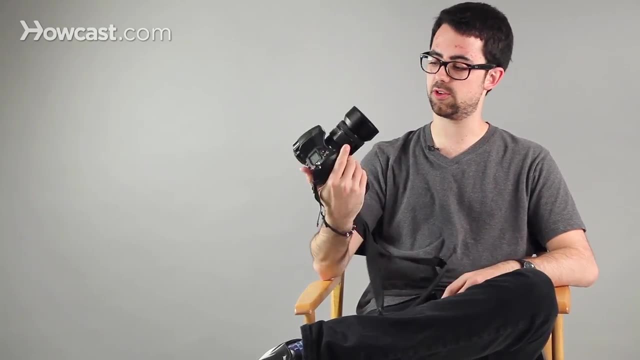 So when you take a picture, what the lens physically does is there's multiple elements inside of this and those elements bring the light in, obviously into focus, and direct it back into the sensor that's behind the mirror. That's how you get your image. 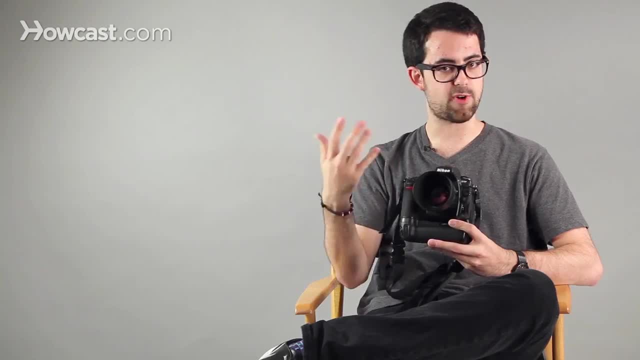 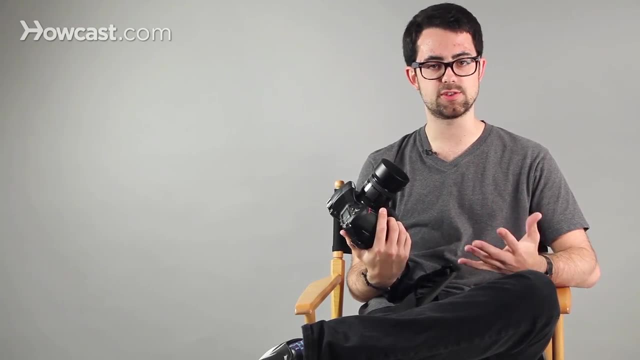 The better the lens quality, the better it looks All right, So the better the image is going to look. Finer lenses, more expensive lenses have just better ground glass with better coatings that help get rid of lens flare, chromatic aberration. and that's just a couple basics. about lenses for digital SLRs. 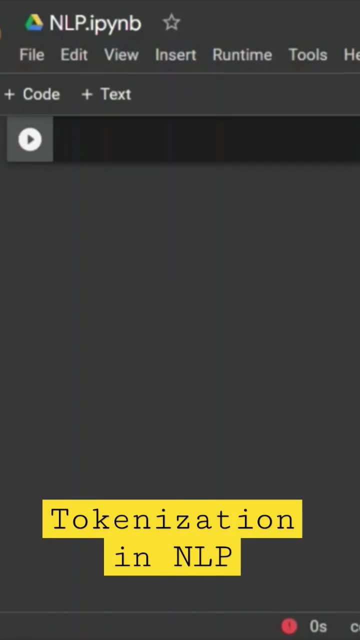 So tokenization is one of the most common tasks when it comes to working with text data. But what does the term tokenization actually mean? So tokenization is essentially splitting a phrase, sentence, paragraph or an entire text document into smaller units. 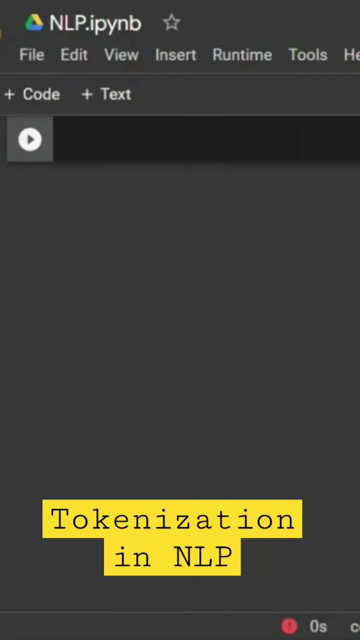 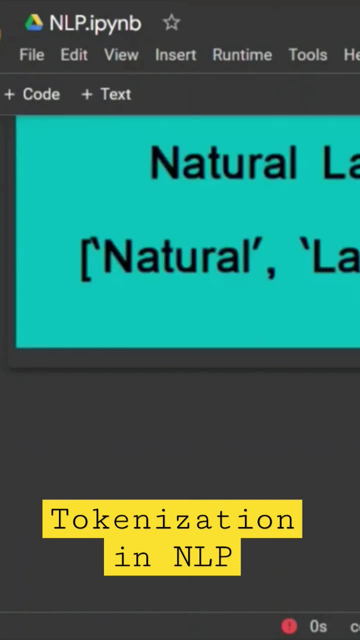 such as individual words or terms. Each of these smaller units are called tokens, So we can look into one particular image. So you can check this image in which the sentence natural language, processing has been broken into three respective tokens. One is natural language and processing. 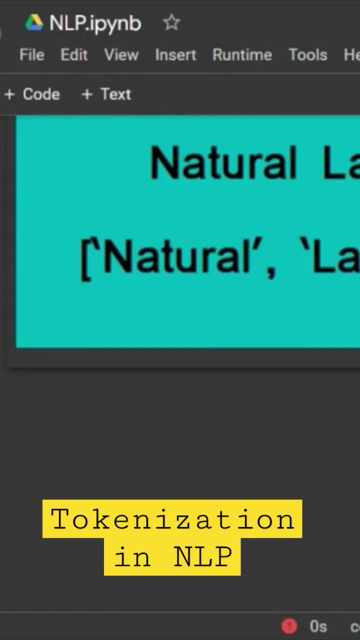 The token could be words, numbers or punctuation marks. In tokenization, smaller units are created by locating word boundaries. Wait, what are word boundaries then? These are the ending points of a word and the beginning of the next word. These tokens are: